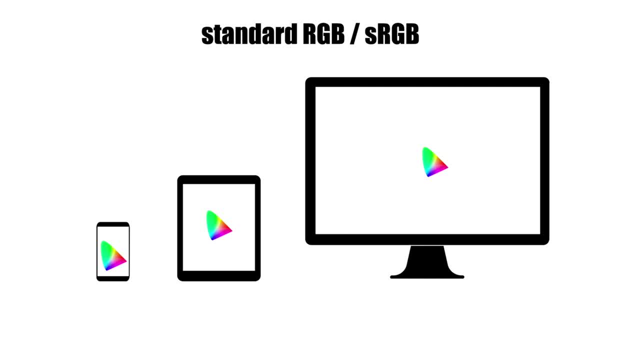 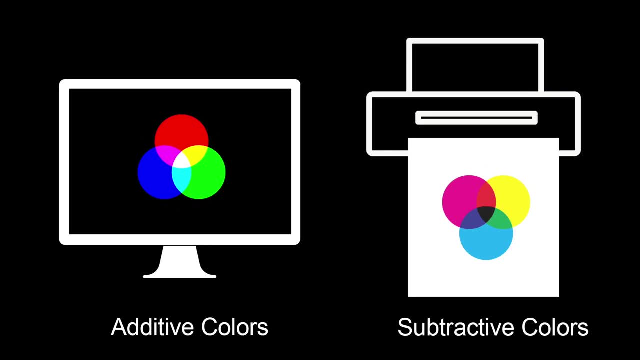 used on different monitors, inkjet printers and the internet. sRGB is still the only color space we use on the web today. When it comes to offset printing press, their inks can't produce the bright and vibrant colors like a backlit display, So a smaller color gamut has to be used, based on a 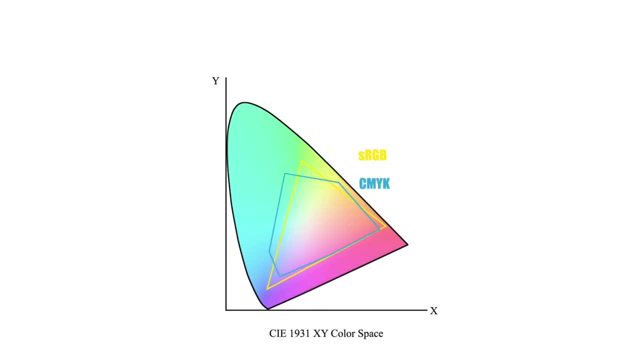 subtractive color model called CMYK. You can learn more about RGB and CMYK and additive and subtractive colors in the video linked above. Now, as you can see, the sRGB color space can't reproduce the entire color gamut of the CMYK color space, Hence the Adobe RGB color space. 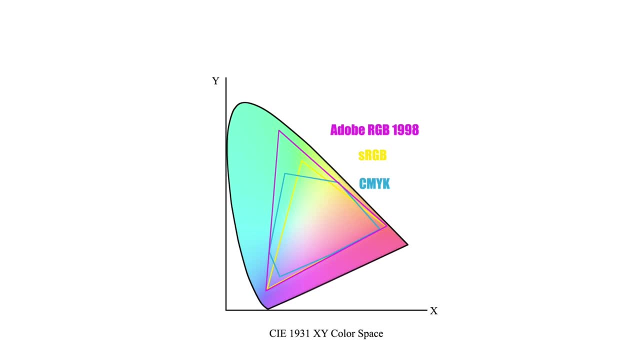 was created by Adobe in 1998, which is much larger than sRGB and it covers the entire color gamut. Another popular color space used in photography is the Profoto RGB, the largest digital color space that was created by Kodak to show all the possible colors in the 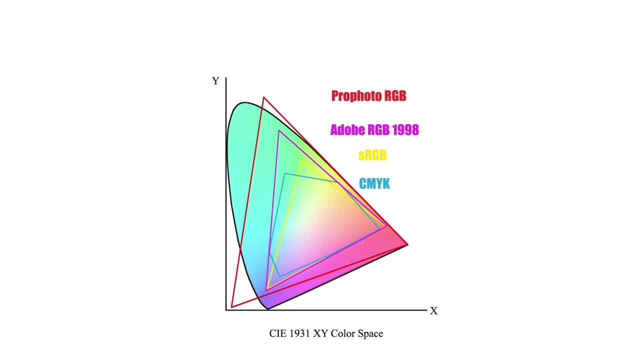 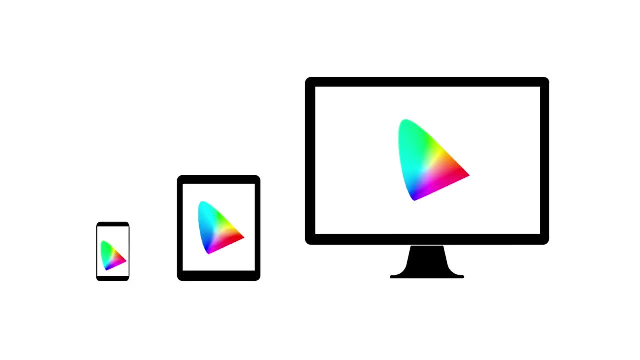 Ektachrome film. So the first thing you notice when you see all these different RGB color spaces is how small the sRGB color space is in comparison. So why would all the devices and web browsers use the smallest color profile? The reason is because there is a gamut limitation with different devices. 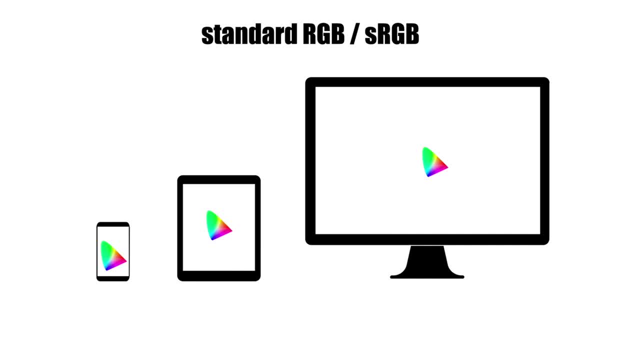 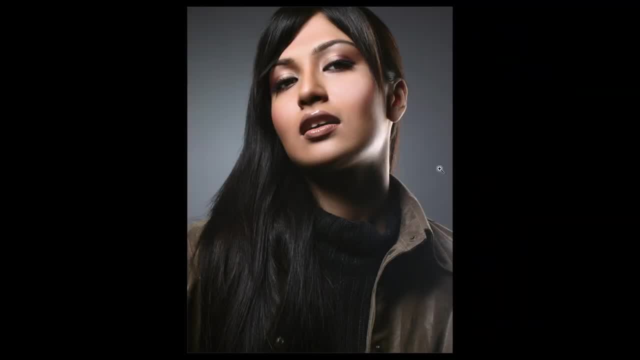 So the standard color gamut has to be small enough to fit in all of them, And sRGB can be handled easily by a 20 year old desktop monitor or the latest smartphone. Most monitors generally use 8 bits per channel, meaning the intensities of red, green and blue. 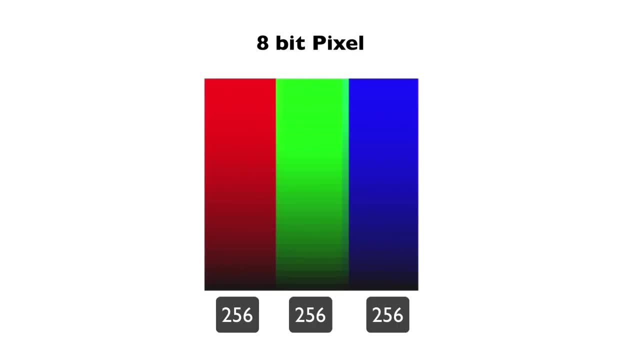 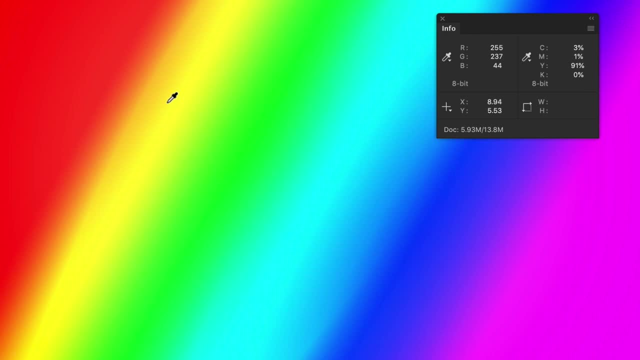 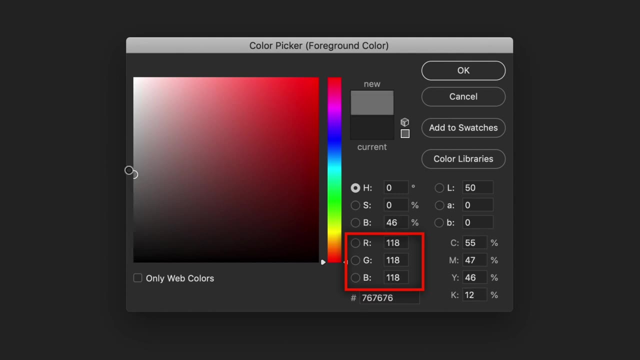 is expressed with an 8 bit value in each pixel, That is, 256 shades of red, 256 shades of green and 256 shades of blue in each pixel. As you might have seen in Photoshop info panel, each color has 4 coordinates within the color space, with RGB values ranging from 0 to 255,. 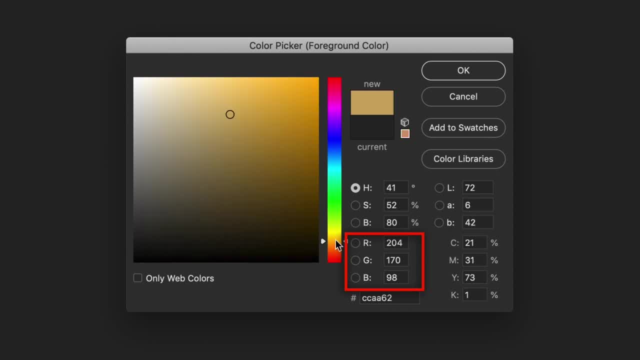 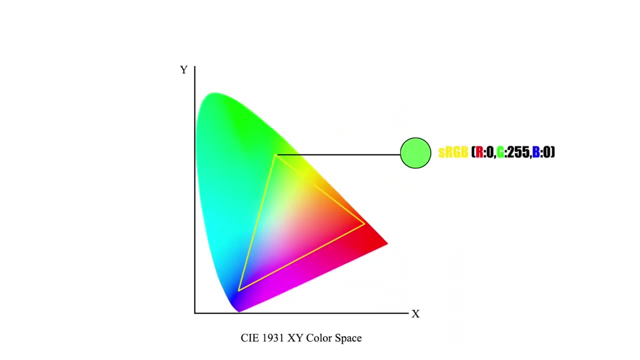 which in total is 256 colors per channel. So every color that you could possibly think of has its own coordinates within the color space. For example, the RGB values of the corner points of the sRGB triangle are defined. so here, like in Photoshop, the purest green point value is: 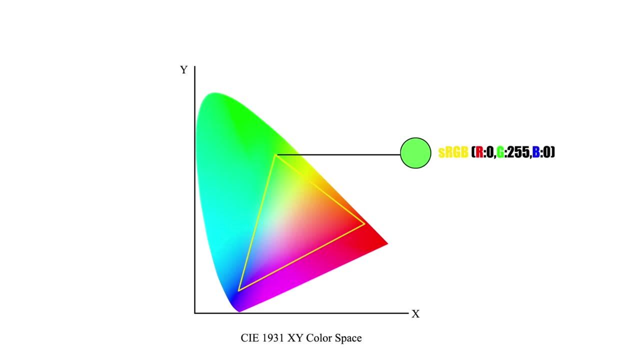 red 0,, green 255 and blue 0.. And these coordinates, or RGB values, are the same for all RGB colors spaces with 8 bits per channel. So even though Adobe RGB has a slightly wider gamut than sRGB, it is still an RGB color. 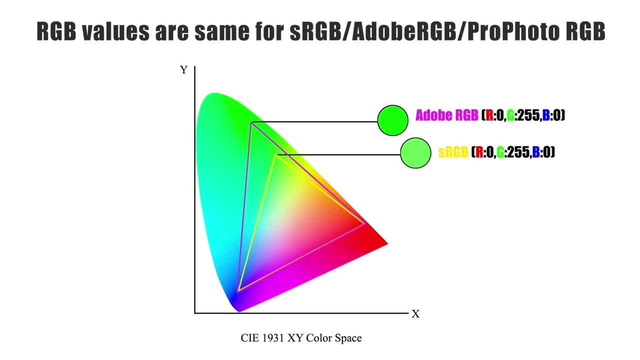 model. so its purest green point here will also be Red 0, Green 255 and Blue 0. But as you can see, it's a completely different green compared to that in the sRGB color space. Now here's the interesting part: when you consider the same purest green point coordinates: 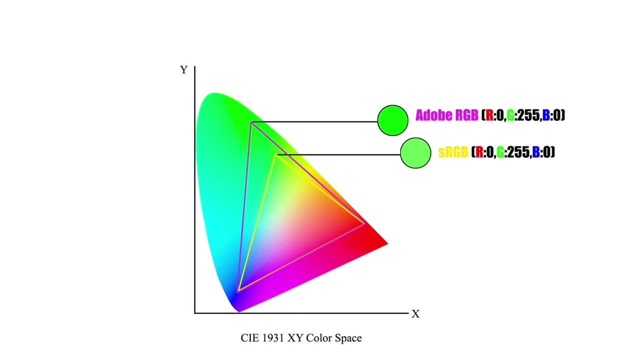 of Profoto RGB, which is also 0 to 550,, you will notice that it is located outside the gamut of the human eye. The out of gamut hue is still green, but what you can't see is the saturation or vibrancy. 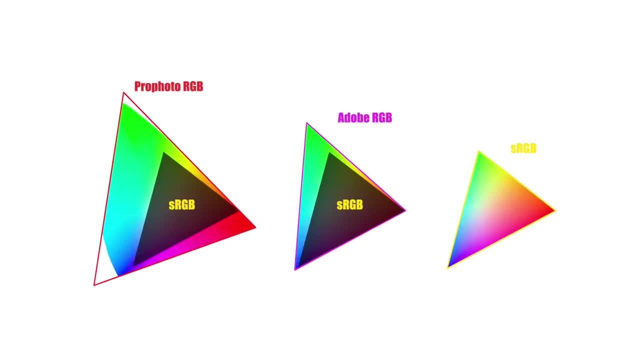 of the green color. So Profoto RGB and Adobe RGB color space do not have more hues than sRGB. they simply have more saturated tint shades and tones, especially in the green and the blue side. Again, if you're confused with these terms, I highly recommend the video on Color Theory. 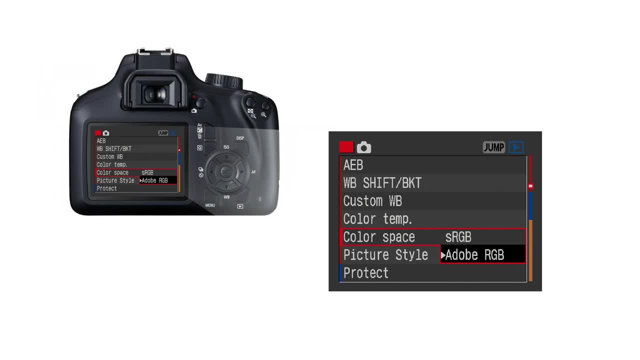 linked above. Now let's move on to color profiles. You might have noticed that cameras usually have an sRGB and Adobe RGB color space option available. Now, these settings strictly apply to a JPEG file. If you shoot RAW, then these settings don't matter. 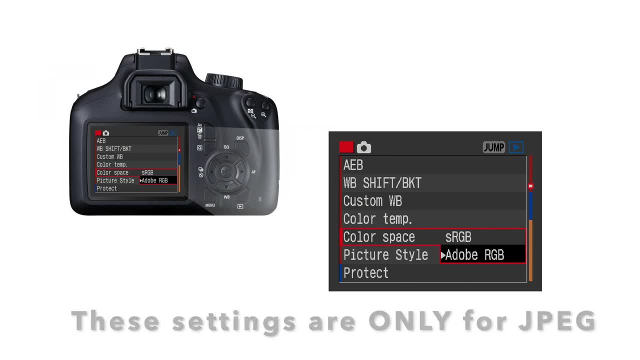 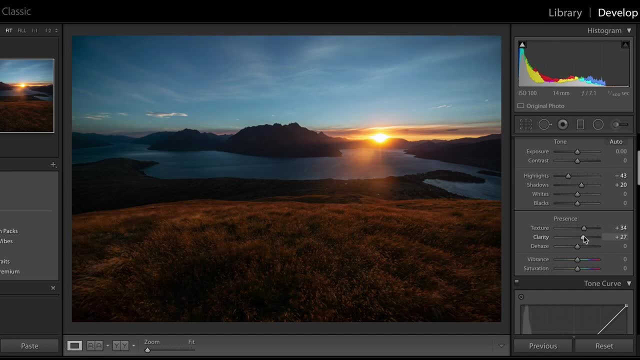 This is because RAW images don't have any color space. it is just RAW data. Lightroom and Camera RAW Converter use a mixture of something similar to the Profoto RGB for processing, but an sRGB for display. Inside there is called the Lightroom Color Space. 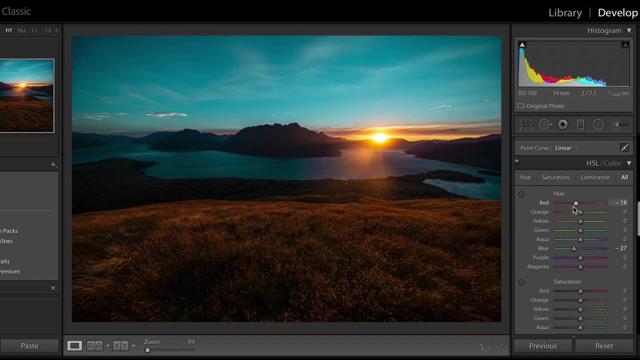 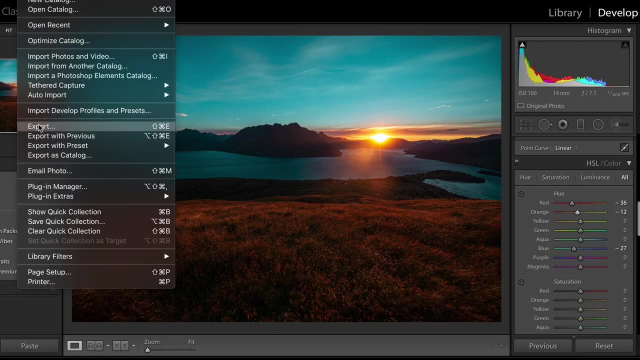 You can see the color space as Melissa RGB named after one of the Lightroom team members. At no point the color values are altered when you edit the RAW photo. Color space has to be assigned to a RAW image during the RAW conversion. When your RAW converter writes out the file, it simply tags the color space by embedding. 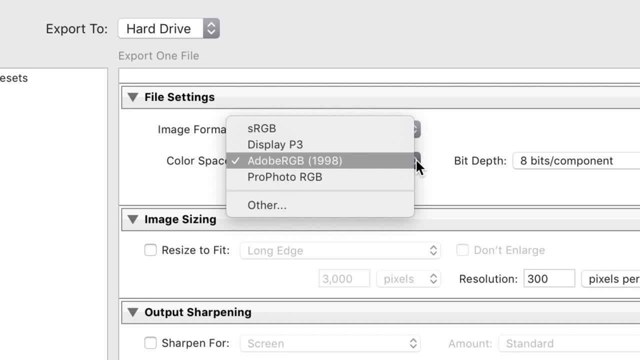 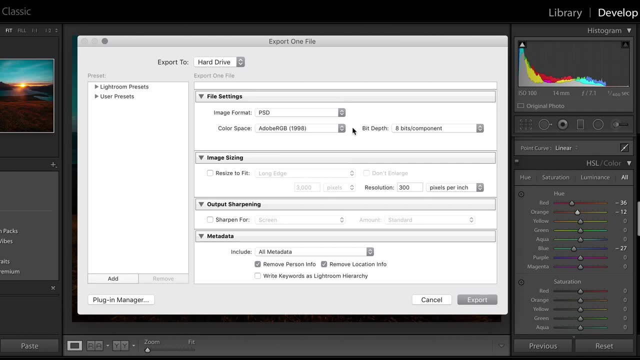 a color profile in its metadata. Color profiles, also known as ICC profiles or ICM profiles, contain the color mapping values of a color space. Think of them as presets of a particular color space. You can also change the color size of a color space. 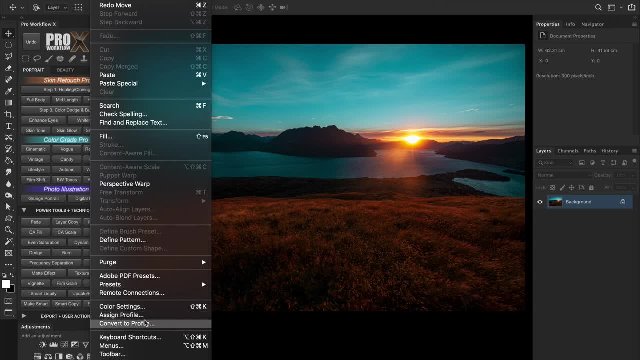 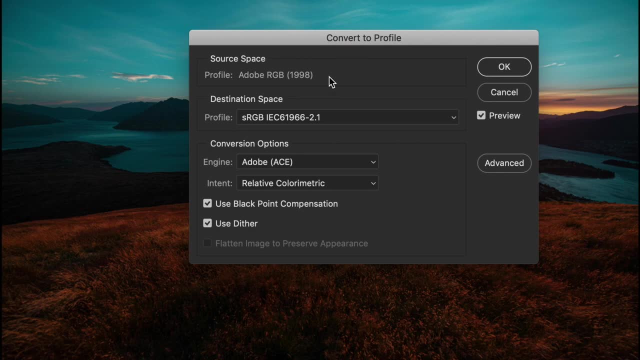 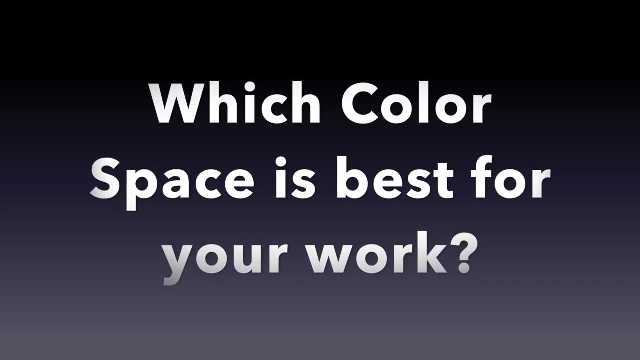 When you open an image in Photoshop, it will map the colors according to the profile assigned during the RAW conversion. This also means that we can remap the colors anytime in Photoshop. Now that you understand color spaces, their gamuts and color profiles, the big question. 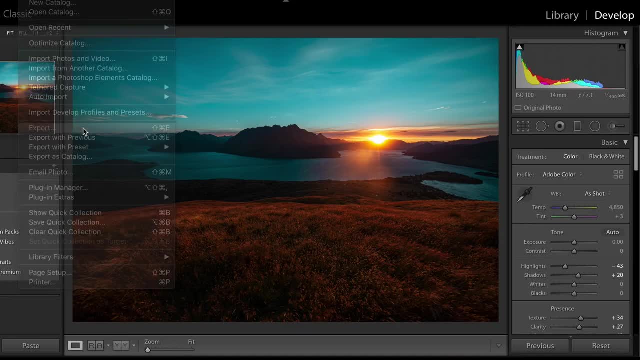 which color space should you use? If you shoot in RAW and edit exclusively within your RAW editing software, simply convert to sRGB for web publishing or Adobe RGB for printing files. If you shoot in RAW and edit exclusively within your RAW editing software, simply convert. 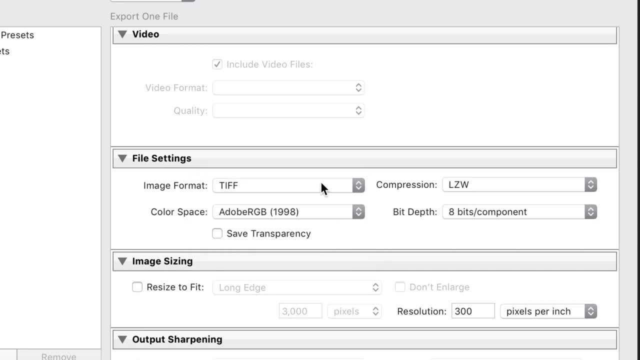 to sRGB for web publishing or Adobe RGB for printing files. This is because the color space is not the same as the color space. Also, the definition of color will be the same as the color space. If you shoot RAW and edit the converted photo with Photoshop, convert in 16 bit Profoto RGB. 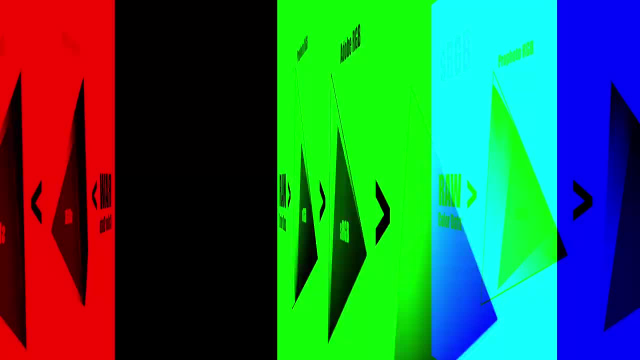 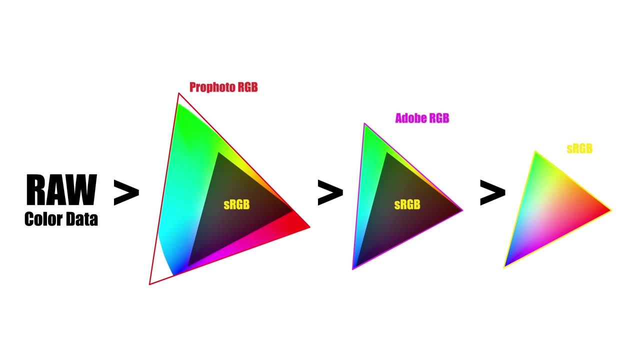 Now, why the Profoto? I'll give you three reasons. First of all, RAW photos often contain colors outside of both sRGB and Adobe RGB color spaces, especially in the high saturation and shadow regions. Profoto RGB ensures that, whatever the actual saturation an image may have, remains un-clipped. 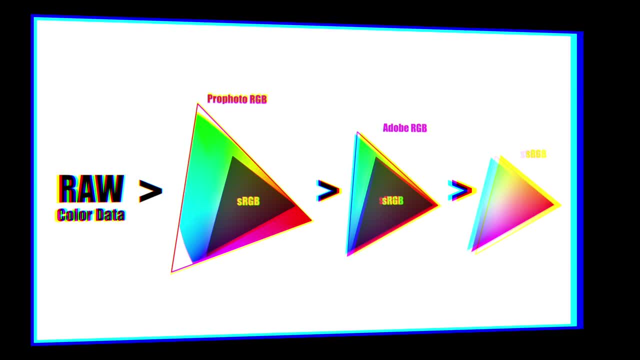 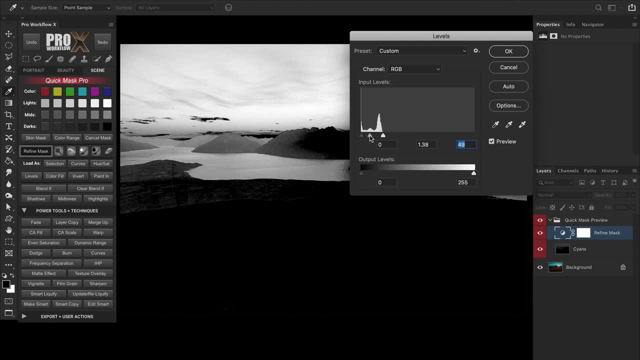 Of course, if your image doesn't have those colors, you won't see much of a difference difference. Second, when you're retouching, you are compressing and pushing all the RGB values around in the image. So the more color data you have, the better your results are going to be. 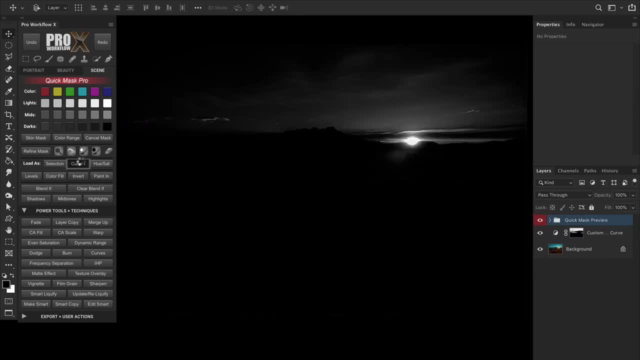 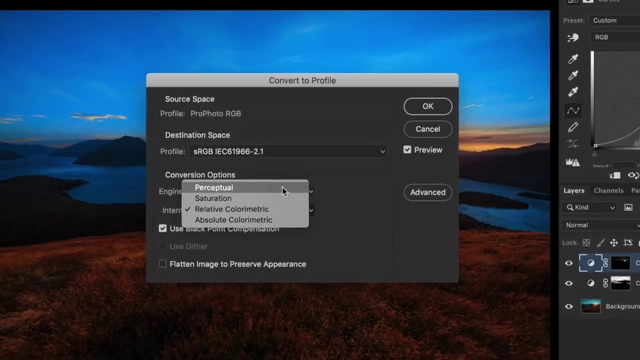 Think of Profoto RGB as a working space or a retouching sandbox inside Photoshop And, when you're done, make the final conversions with rendering intent set at perceptual, as it is the best option for converting from a larger color space to a smaller one. 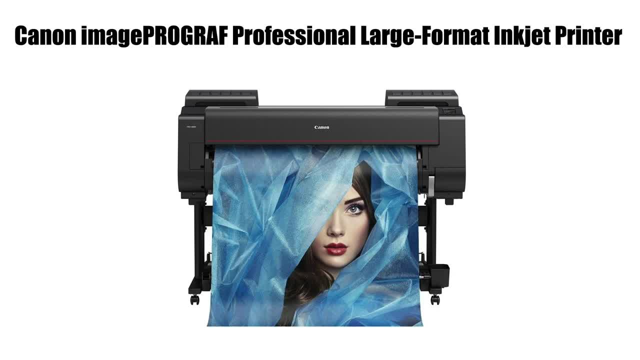 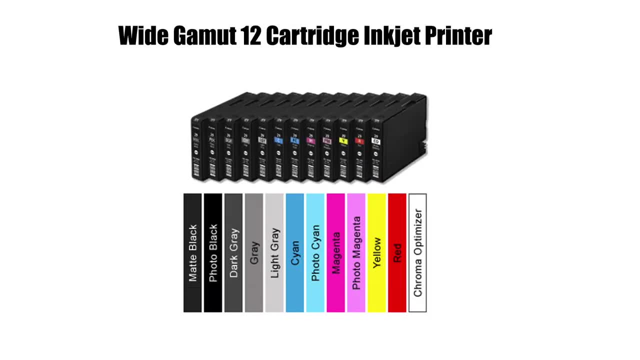 Third, these days, when it comes to inkjet printing, much has changed from the past. Today we have wide gamut high-end printers from Epson and Canon which have up to 12 inks, which exceeds Adobe RGB in some areas. The advantages of Profoto RGB is that it's the only color space that can contain all 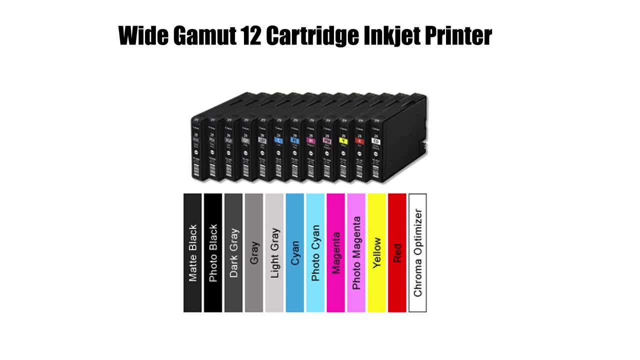 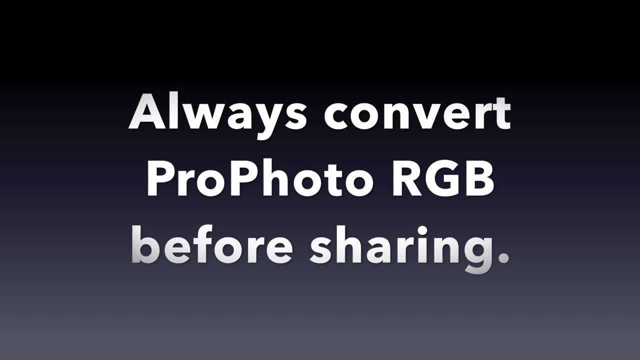 the colors your image can capture in RAW and all the colors that today's wide gamut printers can print. But here are some things that you have to keep in mind while working with Profoto RGB. Just remember that you really don't want to pass a Profoto RGB file off to others who don't understand color management. 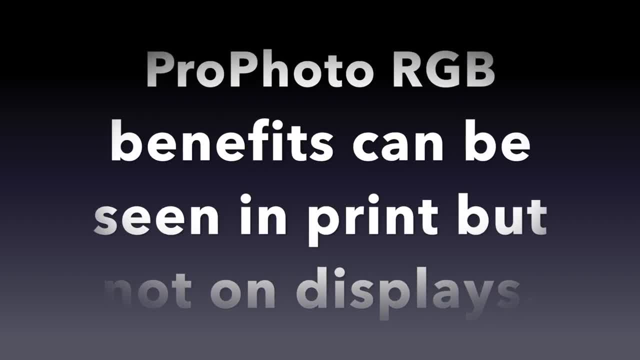 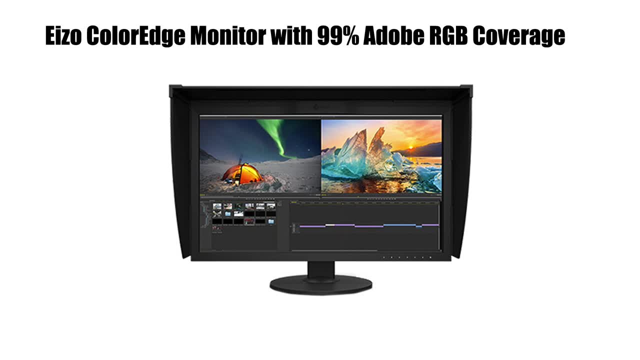 Because, as great as Profoto may sound, there are no wide gamut monitors on the market which display Profoto RGB. For this reasons, many professionals prefer working in Adobe RGB color space, as you will find a monitor that supports up to 99% Adobe RGB, which is fine.